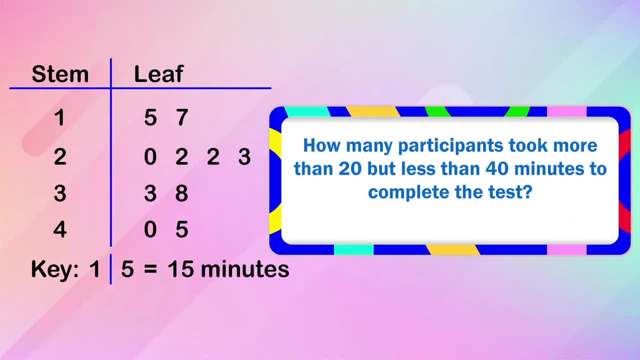 How many participants took more than 20, but less than 40 minutes to complete the test? We have 22,, 22,, 23,, 33, and 38. That makes it 5 participants. How many participants completed the test at the? 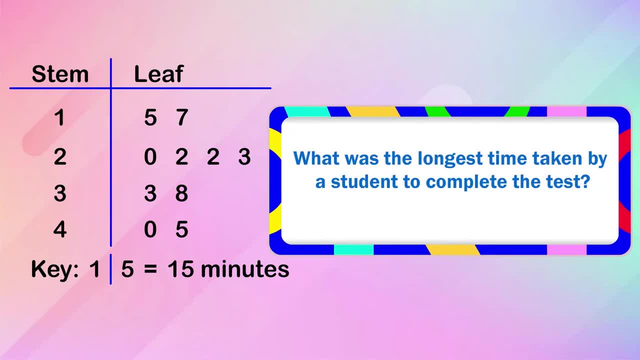 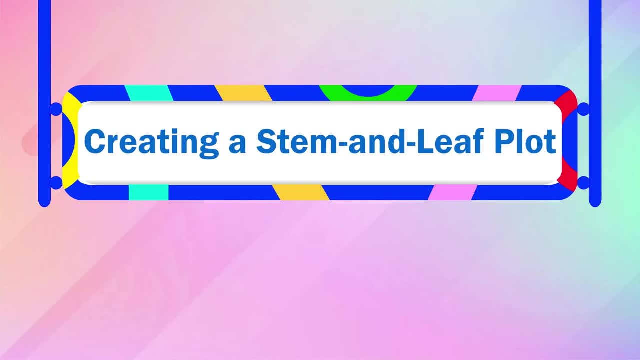 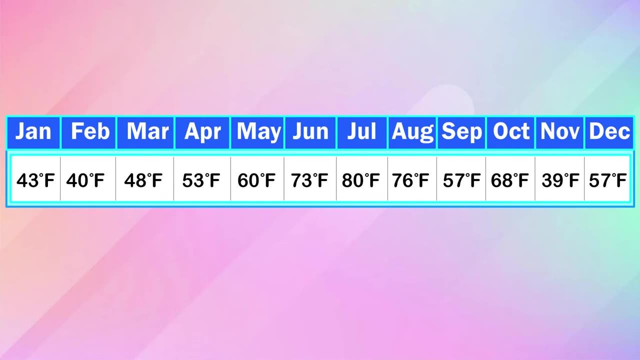 same time. Two: What was the longest time taken by a student to complete the test? 45 minutes. Let's raise the bar and try our hands at creating a stem and leaf plot using the temperatures of a place recorded from January to December. First, we need to arrange the data in. 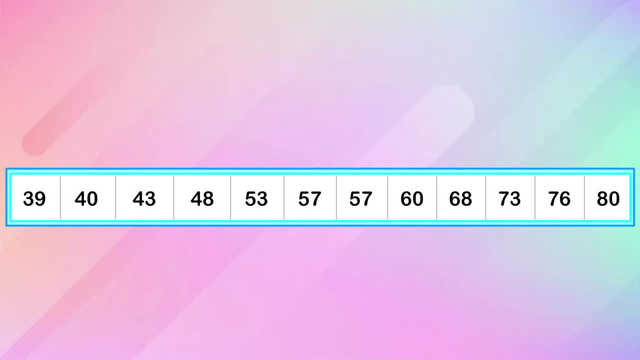 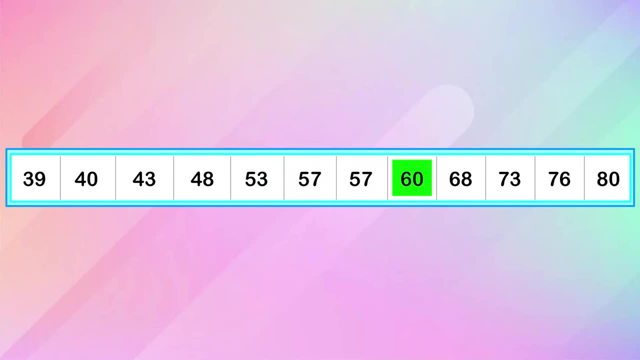 ascending order and determine the highest and lowest temperatures. We have 39,, 40,, 43,, 48,, 53,, 57,, 57,, 60,, 68,, 73,, 76, and 80. The lowest temperature was 39 degrees Fahrenheit. 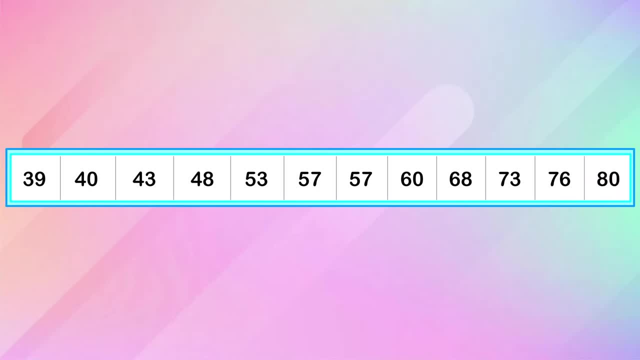 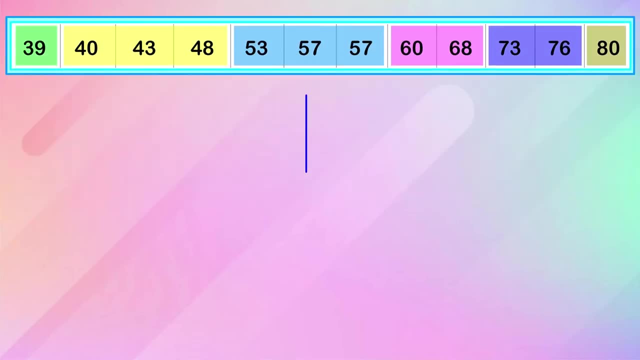 And the highest temperature was 80 degrees Fahrenheit. The next step is for us to identify the stems, Based on the range of 39 to 80, we need 6 stems. We'll draw a vertical line and list the stems on the left side of the line. We'll now fill out the leaves. Let's take a look at our table. 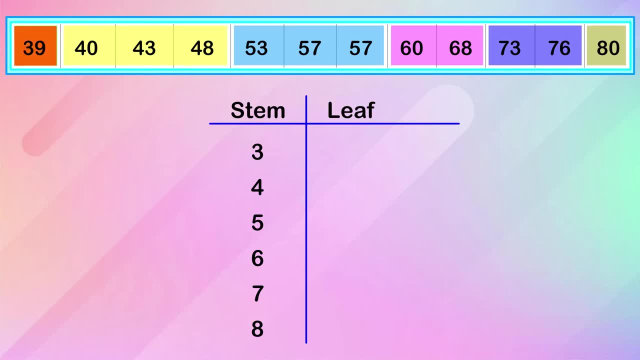 Our first data value is 39 degrees Fahrenheit. We have the stem 3, and we'll write 9 as our leaf. Our next value is 40 degrees Fahrenheit. The stem is 4, and the leaf is 0.. The third value is 43.. We'll add another leaf, 3, to the stem 4.. The next value is 48 degrees. 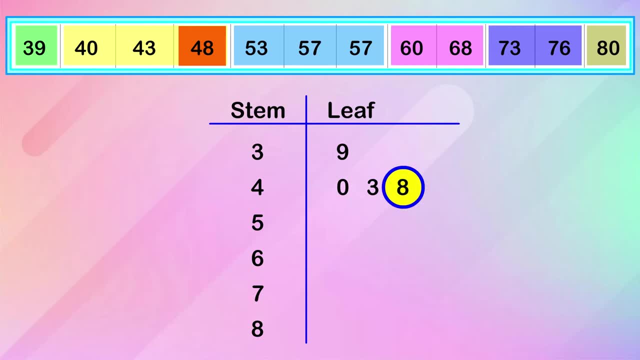 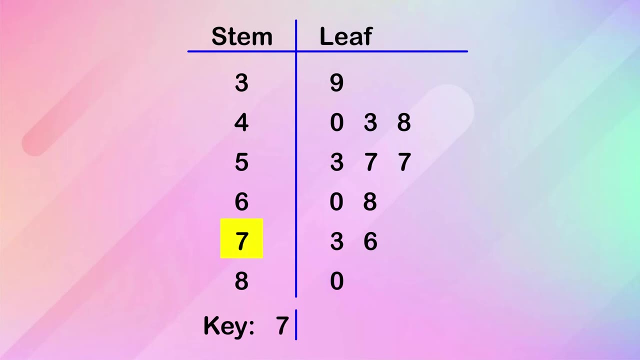 Fahrenheit. We'll add one more leaf 8, to the stem 4.. Our fifth value is 53 degrees Fahrenheit, so we'll add the leaf 3 to the stem 5.. We'll quickly enter the rest of the data. Let's make our key now. We'll pick a value from the stem. Let's take 7.. We'll choose a value for. 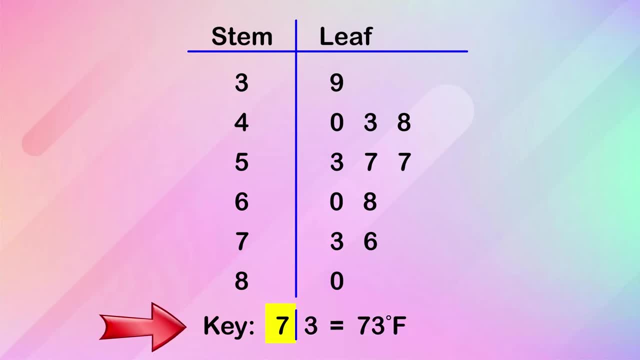 the leaf, Let's take 3.. So This is our key: 7,, 3,, 73 degrees Fahrenheit. So our stem and leaf plot looks something like this: Now that our stem and leaf plot is ready, let's try and answer a few questions.